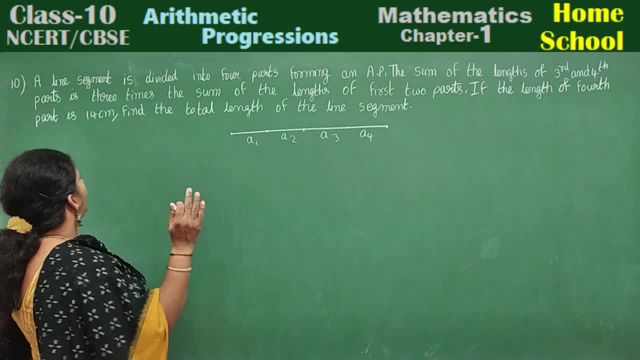 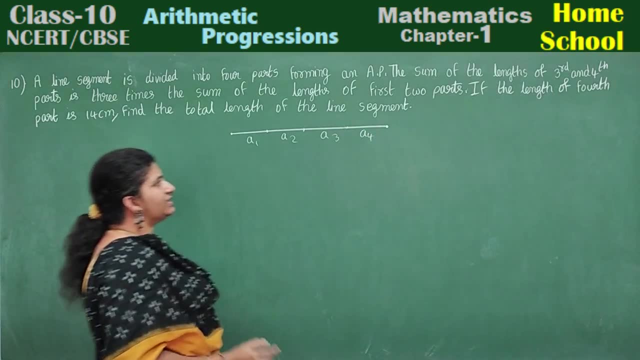 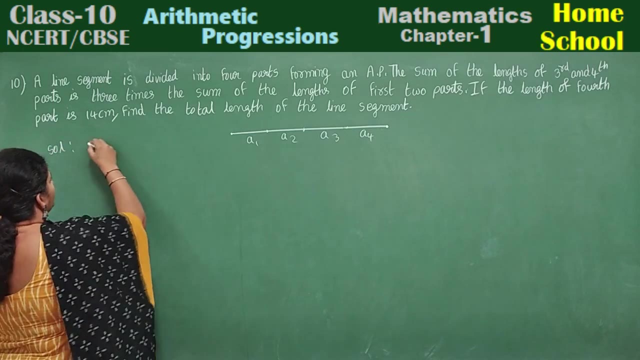 The sum of the lengths of 3rd and 4th part, The sum of the lengths. This length plus this length is equal to. So let me start the solution. We need to write the statement again here That is given. 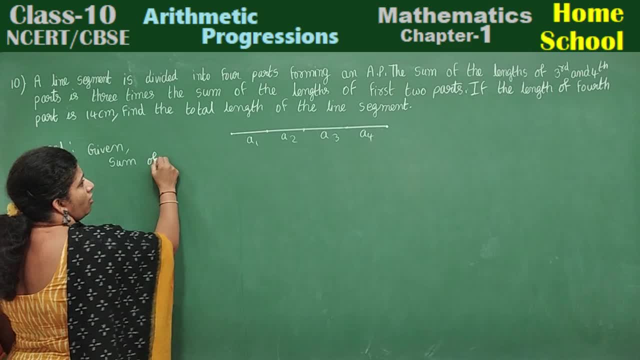 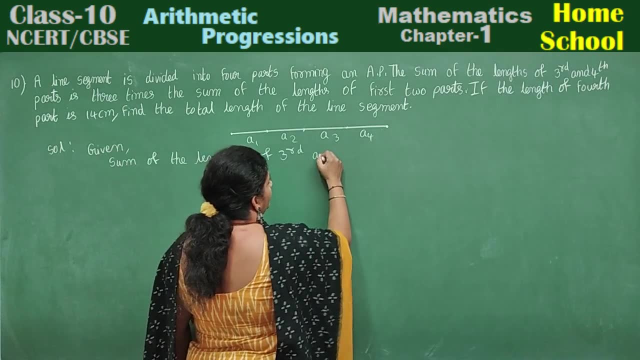 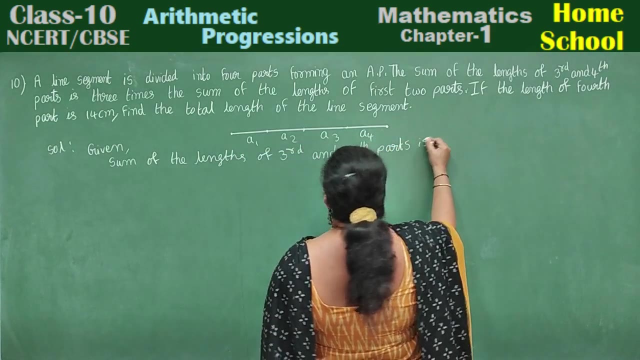 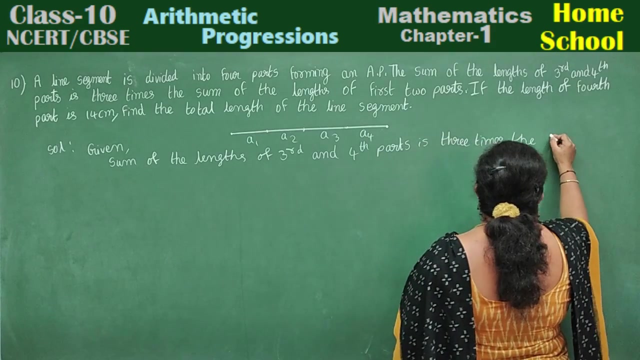 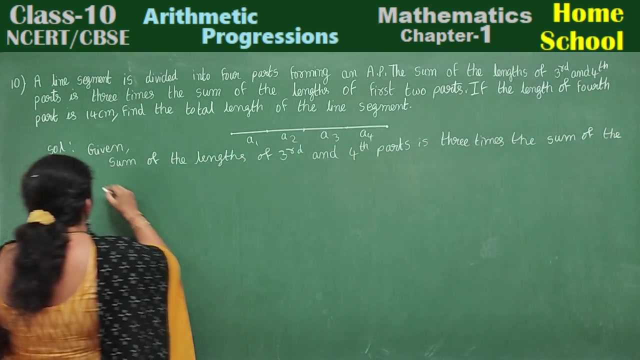 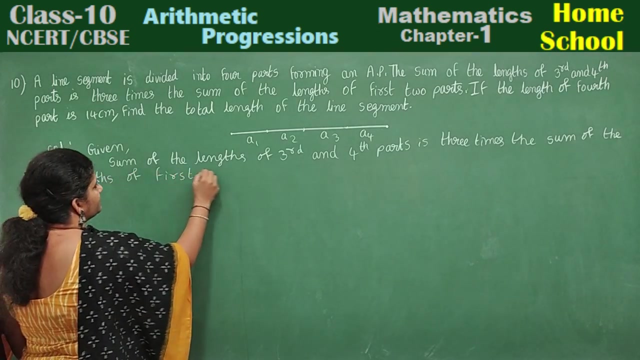 Given Sum of Sum of the lengths of 3rd and 4th part is 3 times the Is 3 times the sum of the Lengths of 1st 2 parts. You can continue. 1st statement also. What is that? Take a line segment. 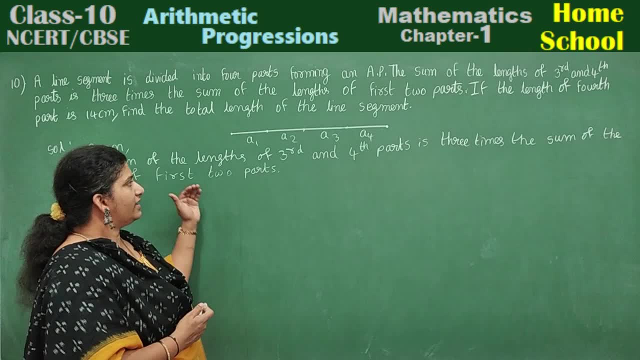 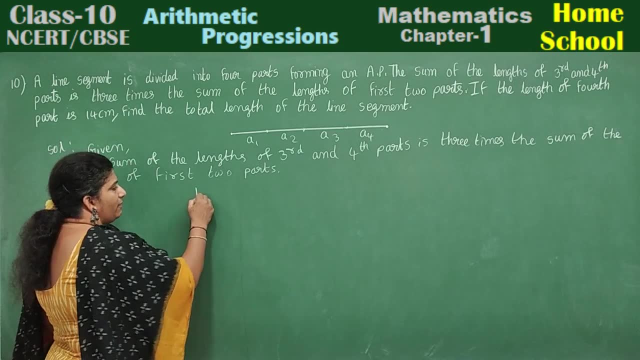 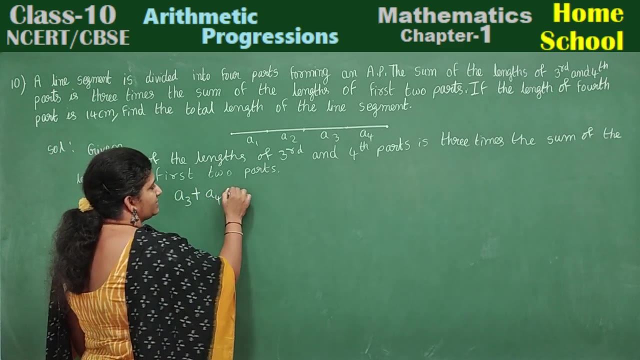 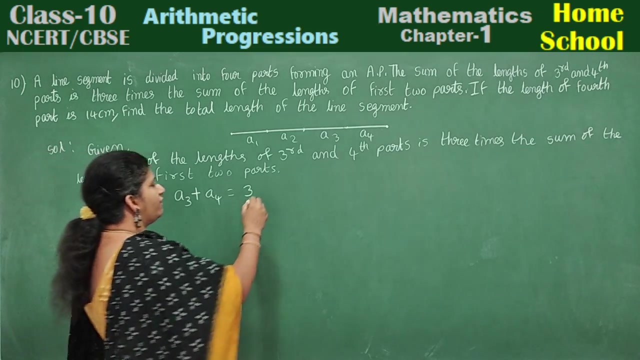 This line segment can be divided into 4 parts and then continue. the statement Sum of the lengths of 3rd and 4th part, Sum plus 3rd part is A3 plus A4. Is Is equal to 3 times 3 times the sum of the lengths of 1st 2 parts. 3 times means 3 in 2.. 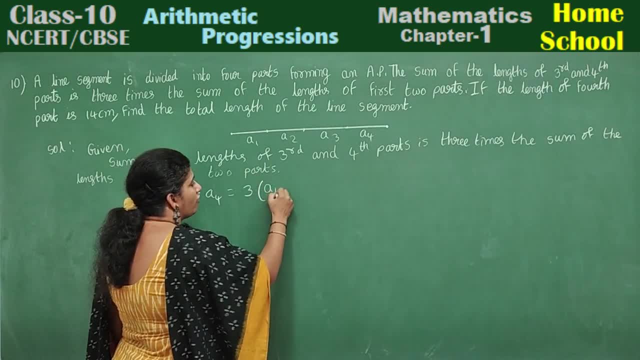 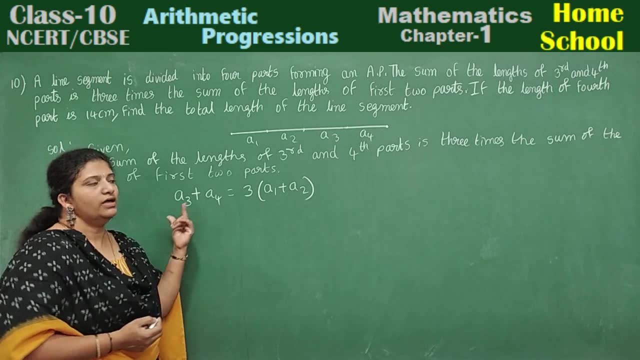 What are the 1st 2 parts, A1 and A2.. Sum of A1 plus A2.. Again, I repeat here: The sum of the lengths of 3rd and 4th part, A3 plus A4, is equal to 3 times. 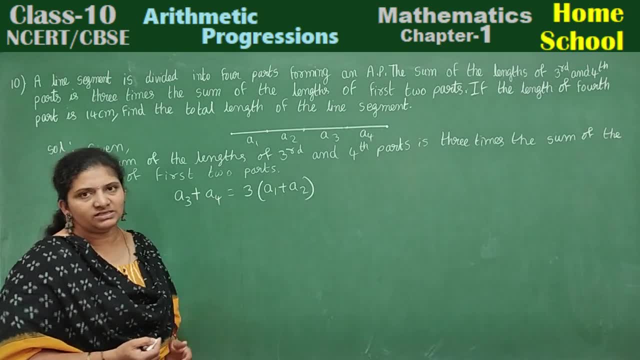 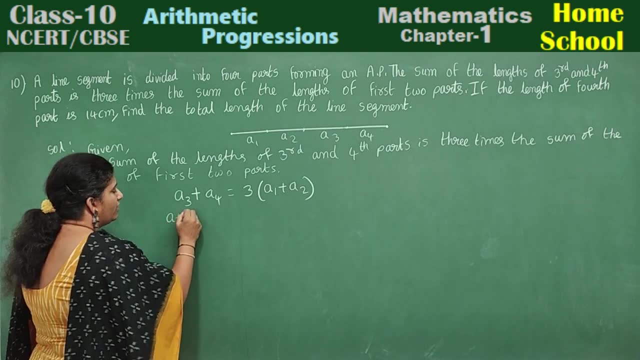 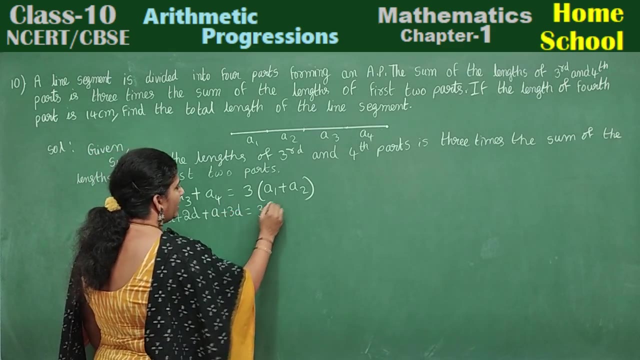 Sum of Sum of 1st 2 parts 3 into A1 plus A2.. You can simplify this and then go with the next statement: A3.. General form: A plus 2D. A4 can be written as A plus 3D. 3 into A1 is nothing but A- A2.. A plus D. 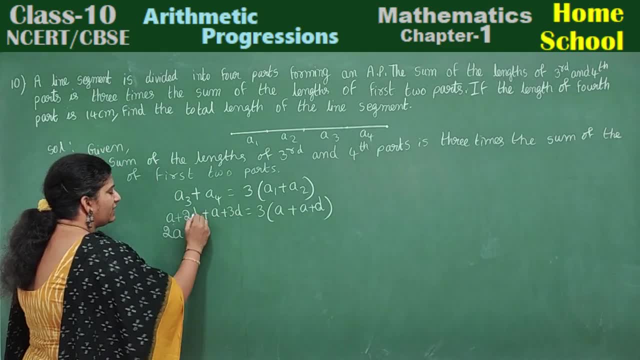 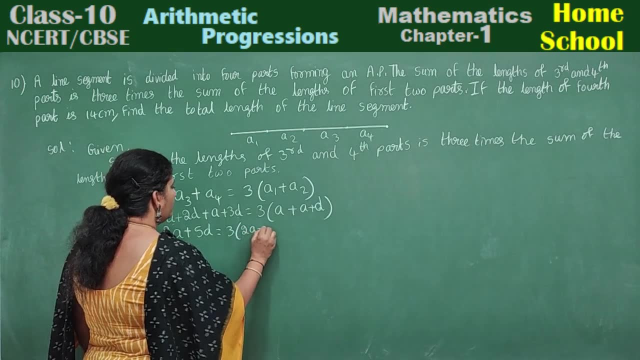 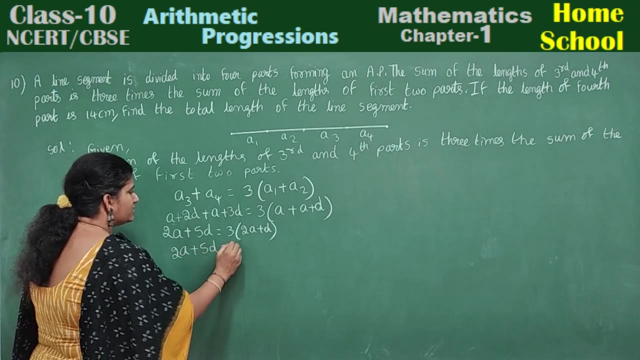 A plus A will be 2A. 3D plus 2D will be 5D. A is equal to 3 into A plus A, 2A plus D. Next step You can remove from brackets: 2A plus 5D is equal to 3, twos are 6A plus 3D. 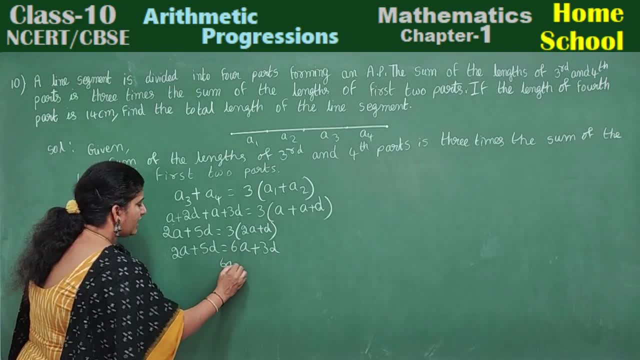 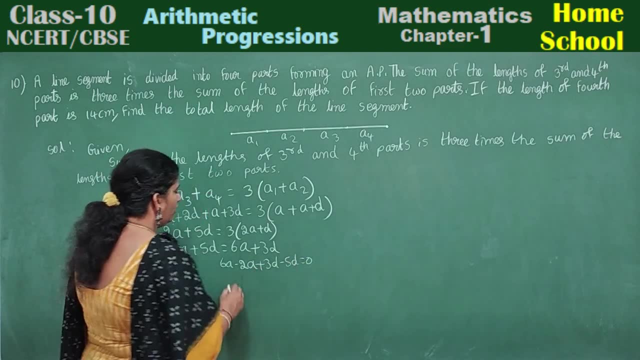 Bring these all this side: 6A minus 2A plus 3D minus 5D, equal to 0.. 6A- 6A- 6A. 6A minus 2D. 6A minus 2D- 6A. 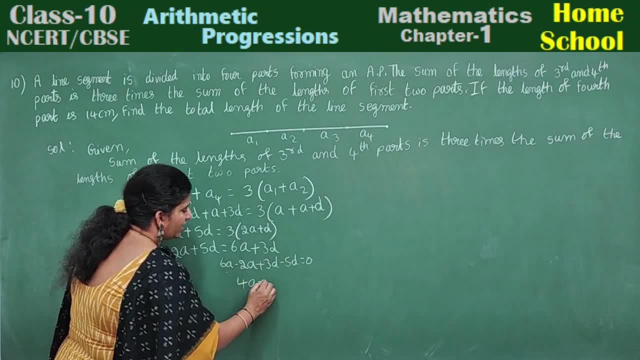 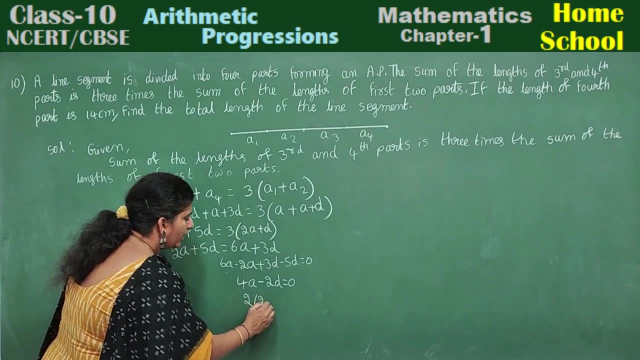 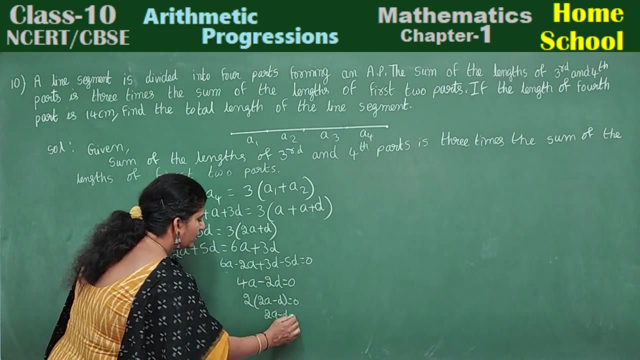 2a will be 4a. 3d minus 5d will be minus 2d, equal to 0.. Take out two common: 2a minus d, equal to 0.. Send this to other side: 2a minus d, equal to 0.. 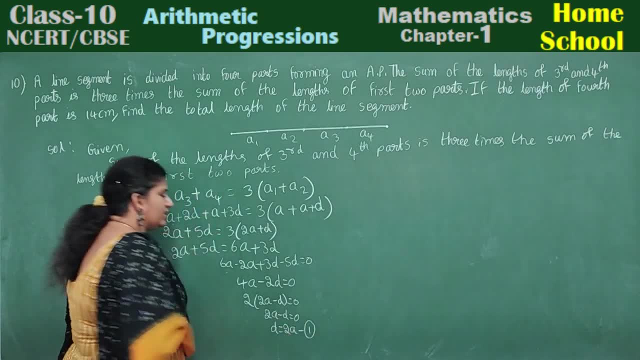 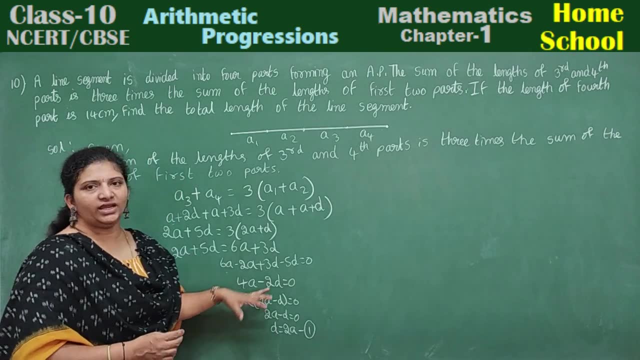 Or d equal to 2a. Mark it first equation. So when I simplify these two, what I got d is equal to 2a. Now read the next point. If the length of 4th part is 14 cm, 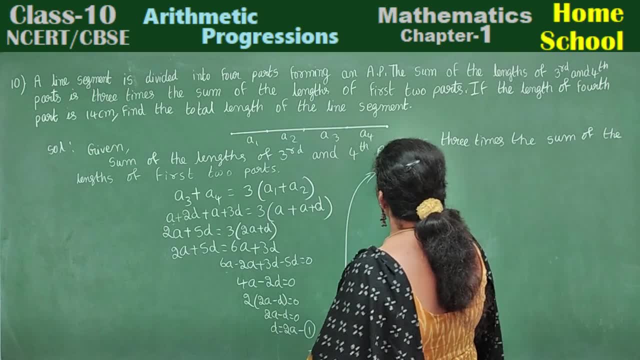 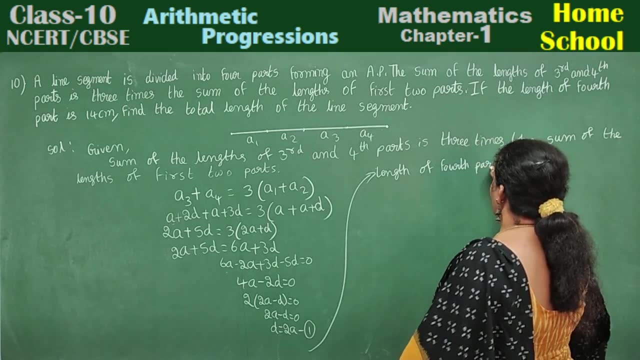 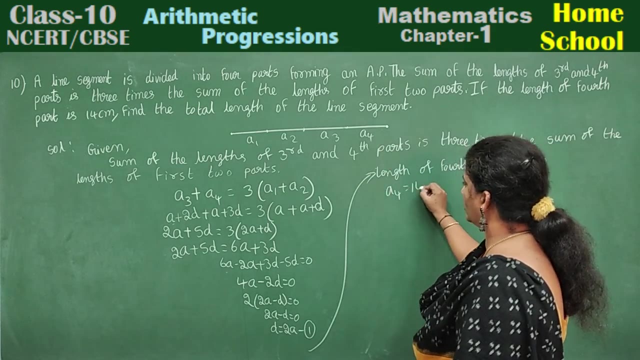 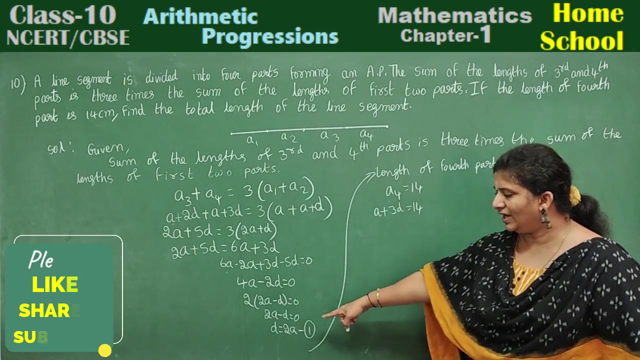 What is given? If the length of 4th part is 14 cm, What is the 4th part? a4 is equal to 14.. a4 general form is a plus 3d is equal to 14.. We know d value. 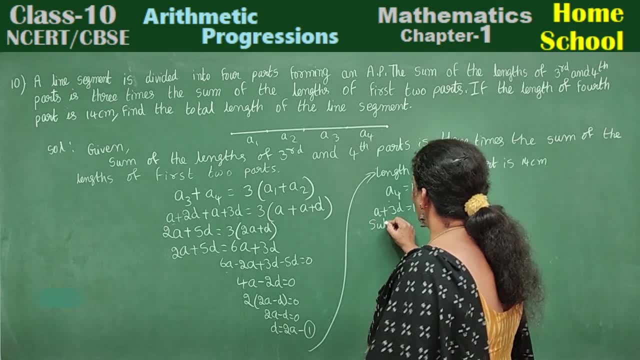 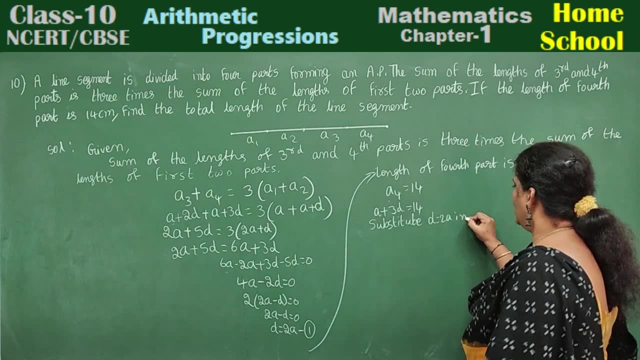 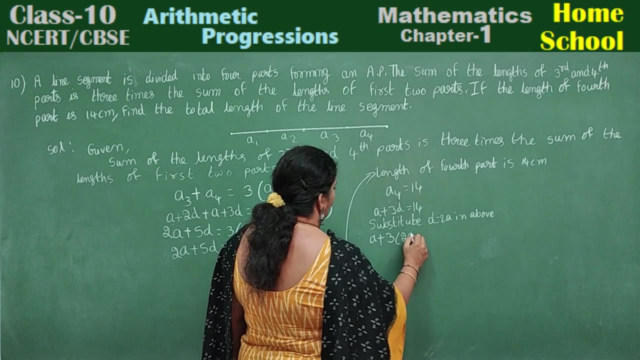 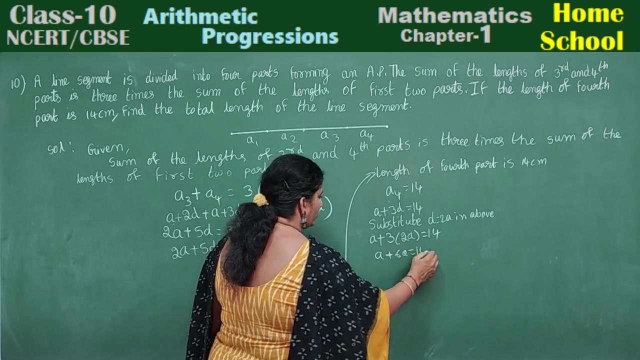 Substitute that d here, Substitute Substitute d is equal to 2a in above. a plus 3 into 2a is equal to 14.. a plus 3, twos are 6a is equal to 14.. 6a plus 6a is equal to 14.. 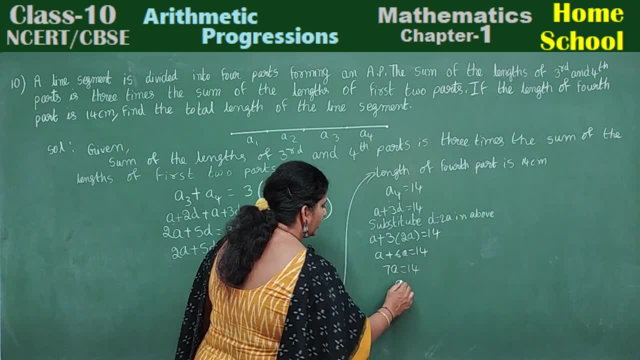 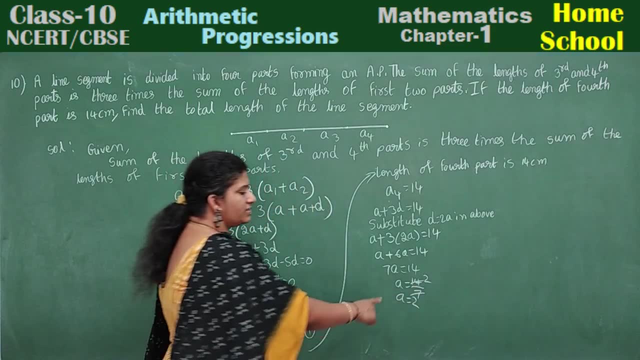 6a plus 6a is equal to 3a. 7a plus n is equal to 7a. 5a plus 6g is mn times 14.. 7a plus 4g is 4g. 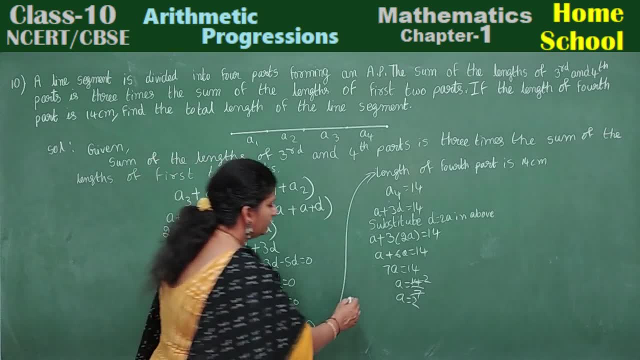 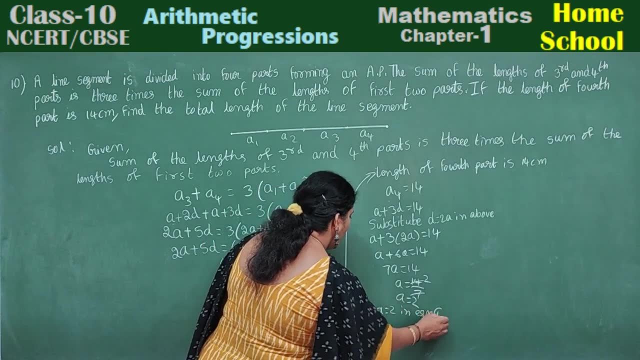 so what we are getting? 7a is equal to 14.. a is equal to 14 by 7.. 2a is equal to 2.. a is equal to 2.. we got this. Then what about d? Substitute a is equal to 2. 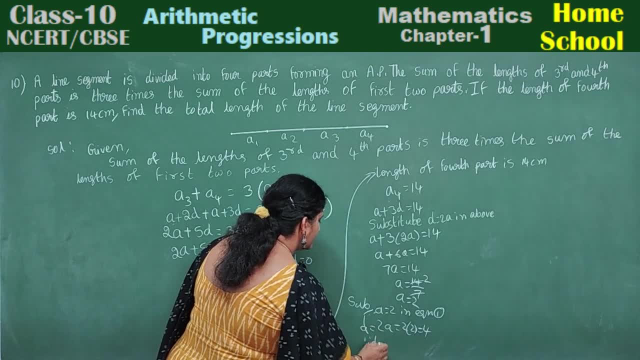 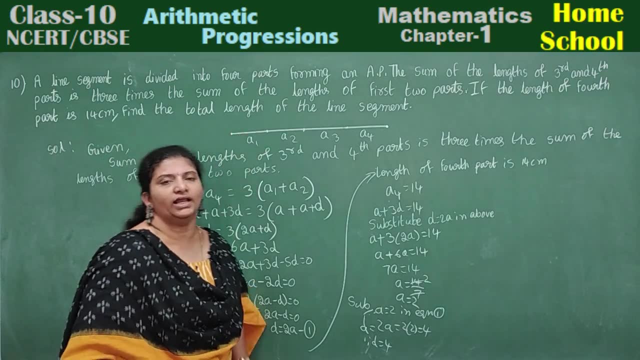 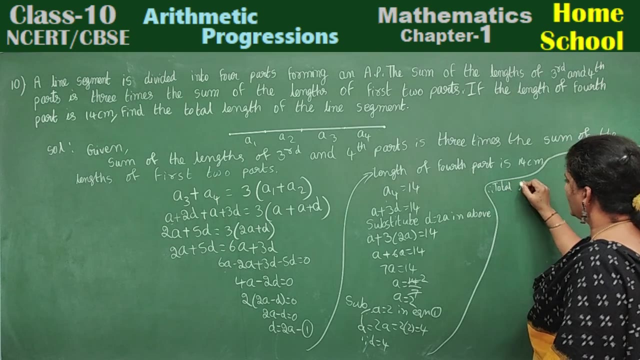 in equation 1.. d is equal to 2a to 4.. And what we need to calculate Find the total length of the line segment. Therefore, total length of line segment, total length of line segment, that is a1 plus a2 plus a3. 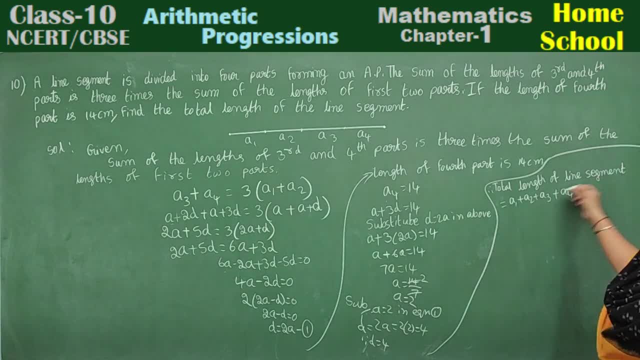 plus a4. that equal to a1 plus a2 plus a3 plus a4.. If you need total length, we need to add all those 4 lengths But a1, write in general form. a plus a2 can be written as a plus d. 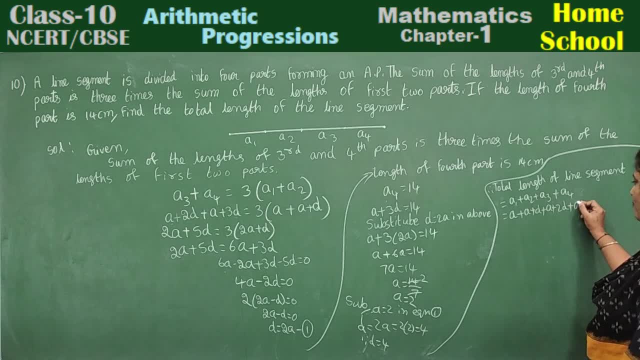 a3 can be written as a plus 2d. a4 can be written as a plus 3d. Now add all this: 1, 2, 3, 4, 4a plus a1 plus a3 plus a4.. 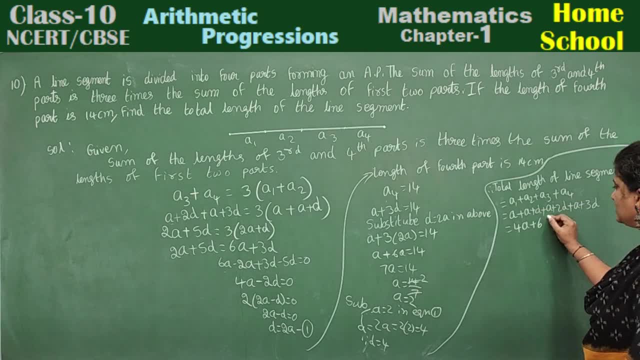 2D plus D plus 3D will be 6D. Okay, Now substitute A value and D value. A is 2.. 4 into 2 plus 6 into 4.. Since A is equal to 2 and D is equal to 4.. 4- 2's are 8.. 6- 4's are 24.. 24 plus 8 it will be. 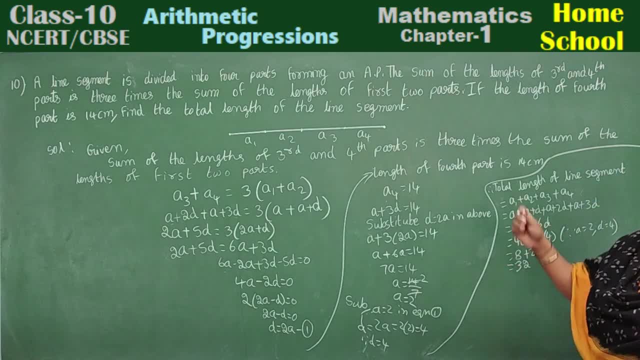 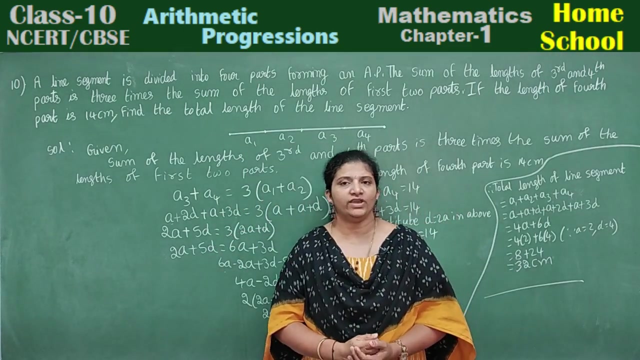 32.. Length: 32 centimeters. Why centimeters? They have given this part as 14 centimeters. Therefore length. Therefore, the total length of line segment is equal to 32 centimeters. We need to end up this problem with that line. The same problem we can do in another way, That is, any 4. 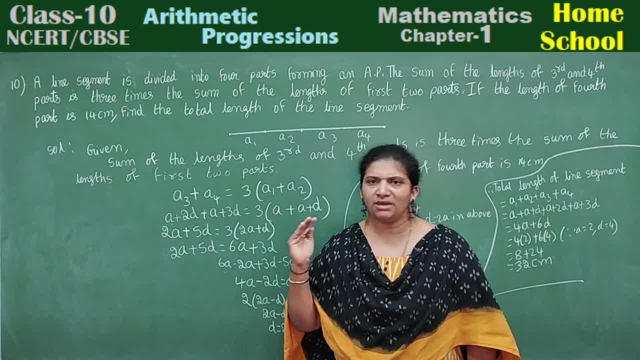 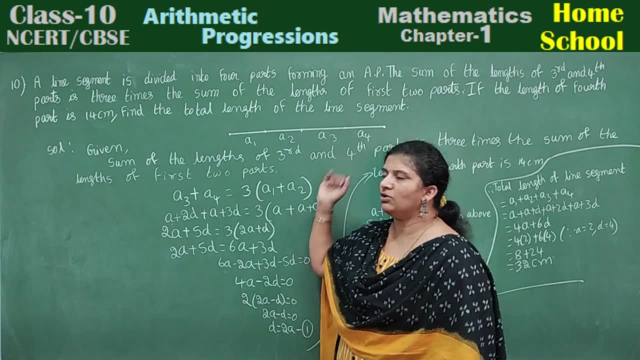 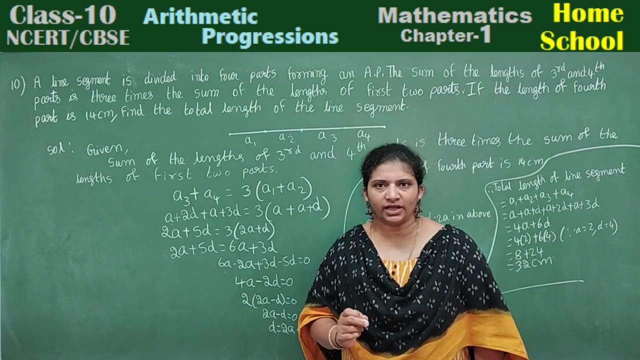 terms, 4 terms. This means what we can remember: A minus 3D, A minus D, A plus D, A plus 3D. In that manner also we can proceed the problem Any way you can do. This is your 10th problem, 9 problems already.